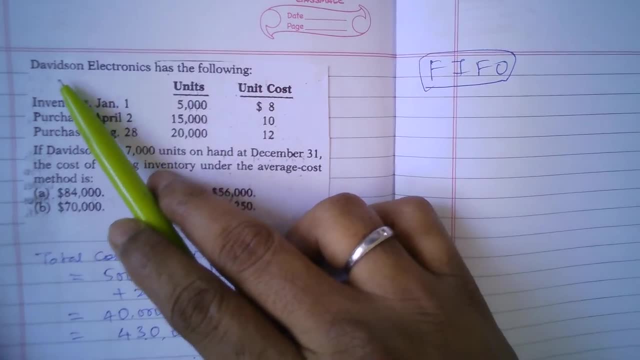 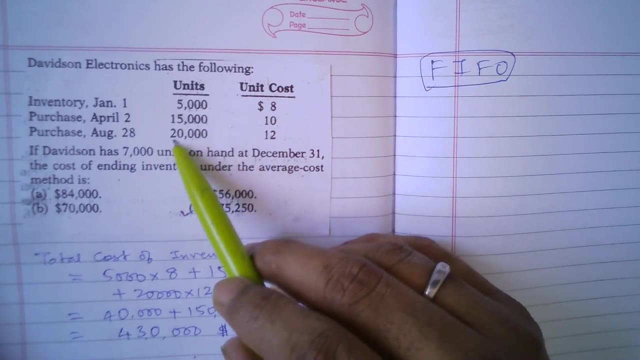 what we are doing here is the company Davidson Electronics purchased, had an inventory on January 1st of 5000, purchased 15,000 on April 2nd, purchased 20,000, now at different costs. now it has 7,000 units on hand at December 31. now which are the 7,000 units? are the 7,000 units which were? 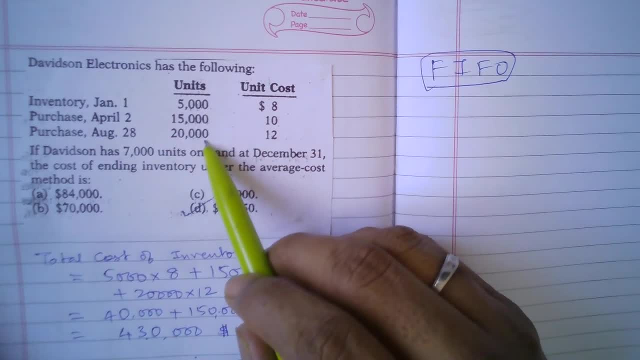 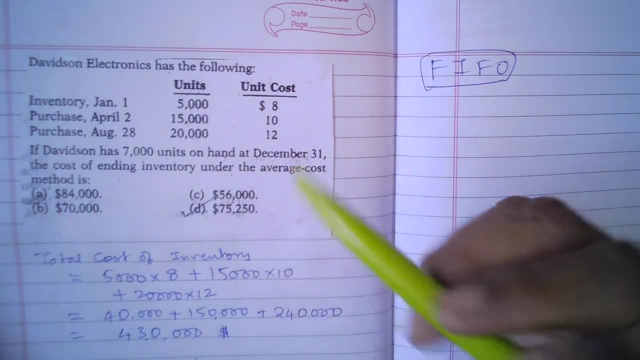 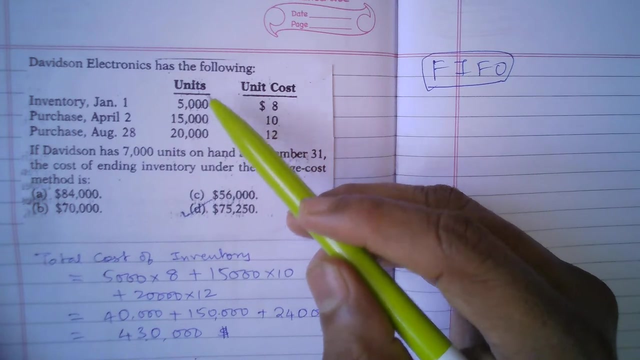 purchased which were at the original inventory or the last one recently purchased units on August 28th. so in the FIFO principle what it says is: first in, first out. that means you will sell the inventory which was first you purchased. that means the 5000 inventory is sold 15,000. 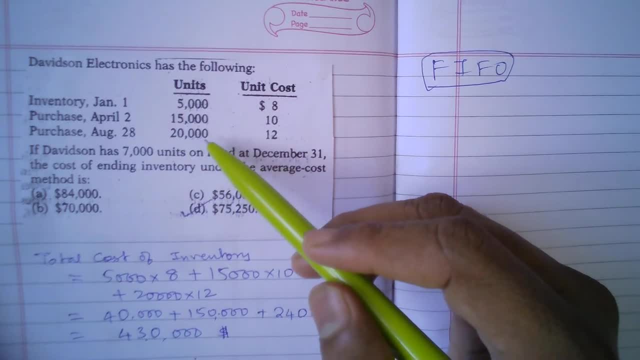 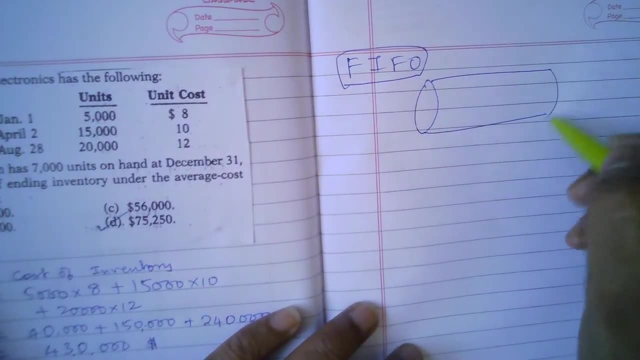 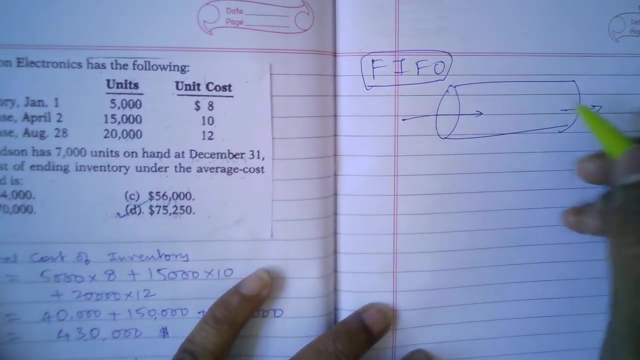 inventory is sold. only after that you will start selling the 20,000 inventory. so first in, first out is something like if you consider it as a pipe, so in this, whatever enters into the pipe, so first go out, okay, so what? what was the first entered into the pipe? so here I will just make some circles. 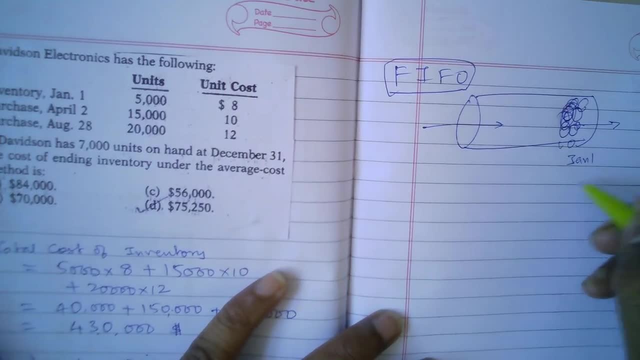 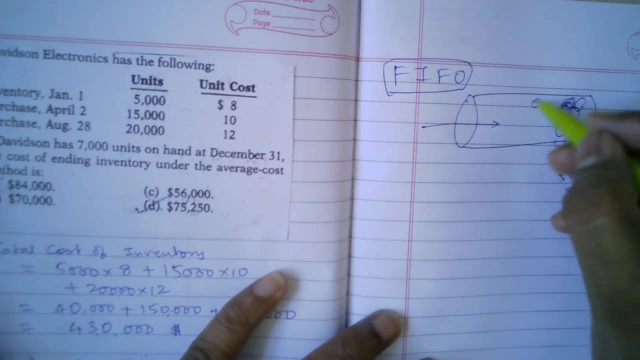 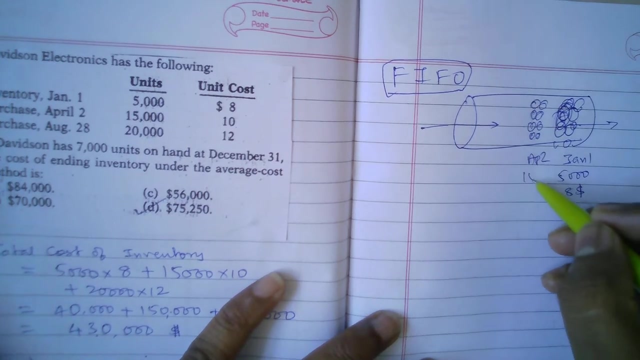 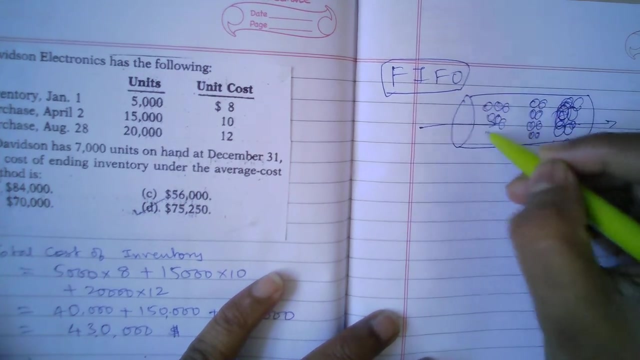 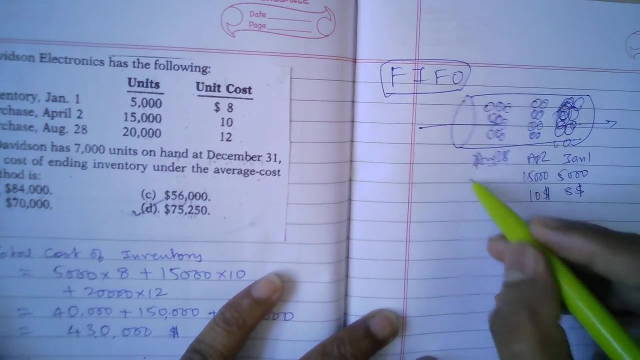 okay, so this is the inventory purchased on Jan 1st: okay, and 5000 units and cost of $8. next, the items that were purchased were on April 2nd and then 15,000 units and then the cost was $10 and Items purchased were on August 23rd and then next the items purchased were on August 28th and there are 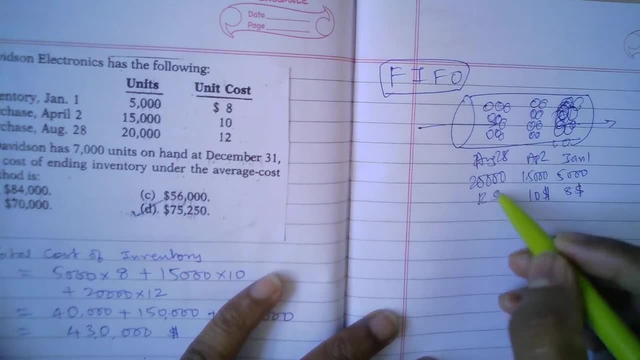 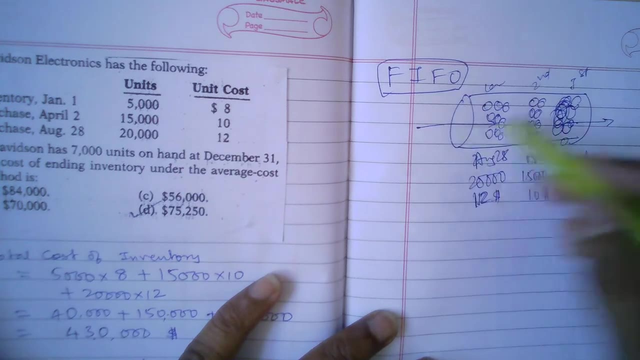 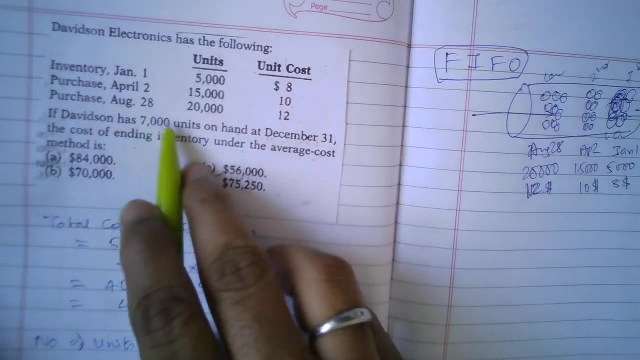 20,000 items and the cost was $12. now which one entered? the first, the first to this is the first, this is the second and this is the last. so first in, first out. that means these are sold. so how many are sold? inventory balance: inventory is only 7,000. that means all these are sold, all these. 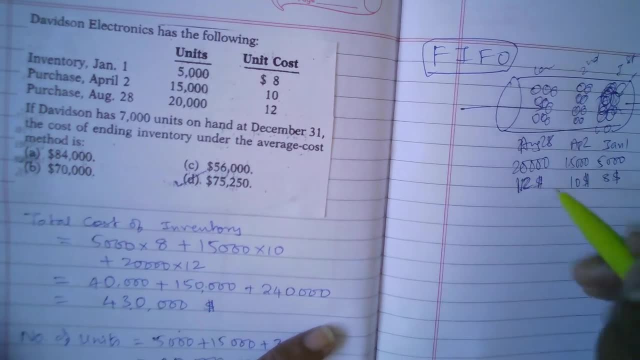 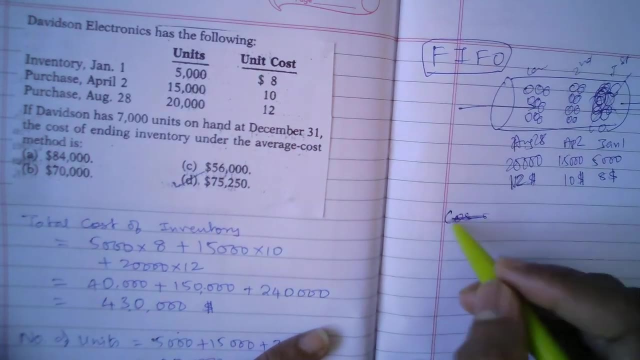 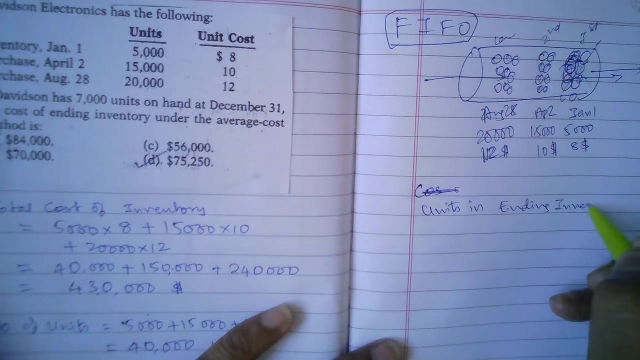 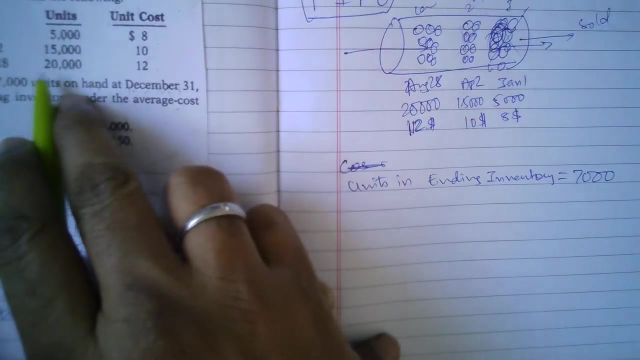 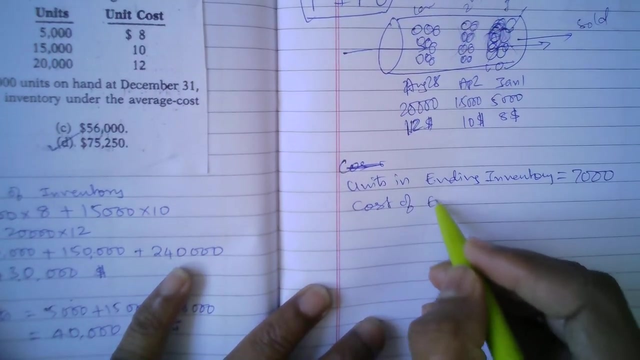 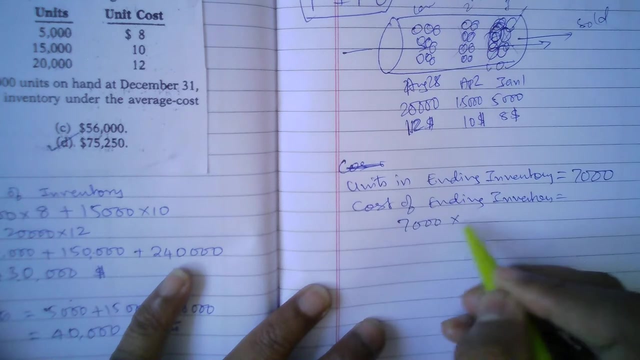 are sold. only out of this 7000 are remaining. So you simply start from the bottom and take the unit cost. So cost units in ending inventory is 7000.. So then out of 20000, 7000 is less than that. So therefore you can directly take cost of ending inventory. simply is 7000 multiplied. 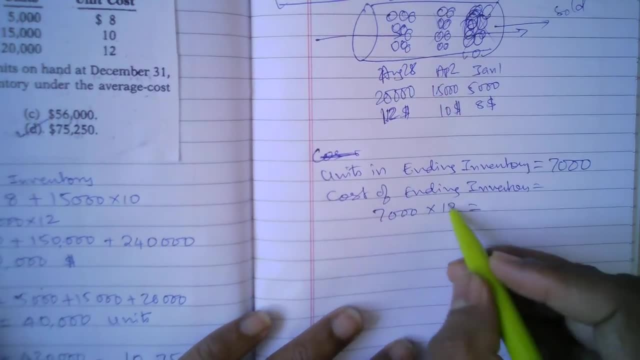 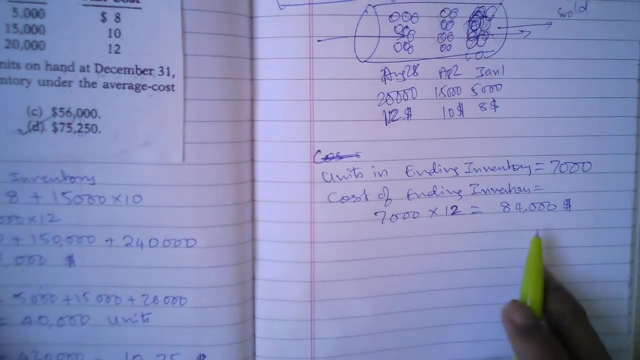 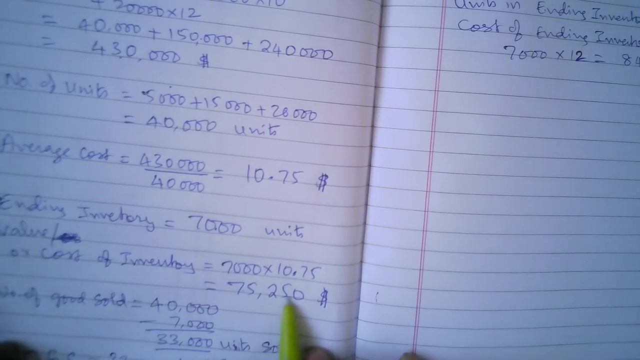 by 12.. So you will get 7 into 12, $84000.. So the cost of ending inventory is 84000.. Earlier, what was the cost of ending inventory? The cost of ending inventory was 75000. So the cost of ending inventory was 84000. So now it increased from 75250. it increased to 84000. 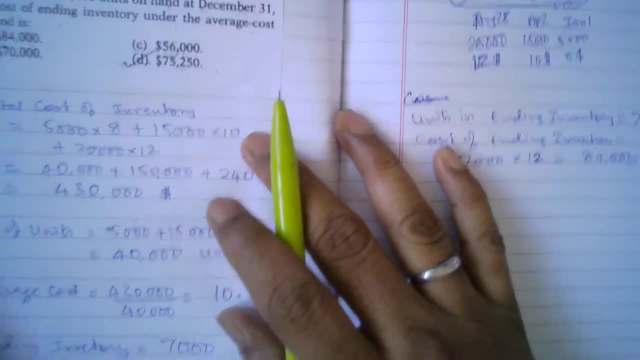 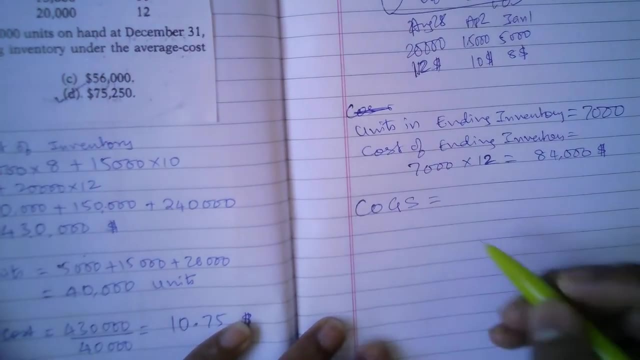 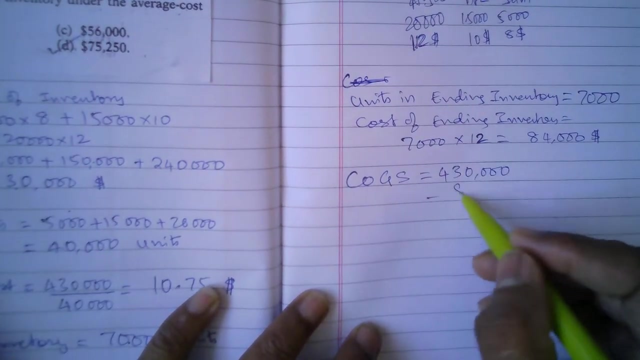 So the cost of the inventory has increased, So at the same time. so now if you want to say cost of goods sold here, you simply take the total cost of inventory, that is 430000 minus 84000. So then you will get the cost of goods sold. 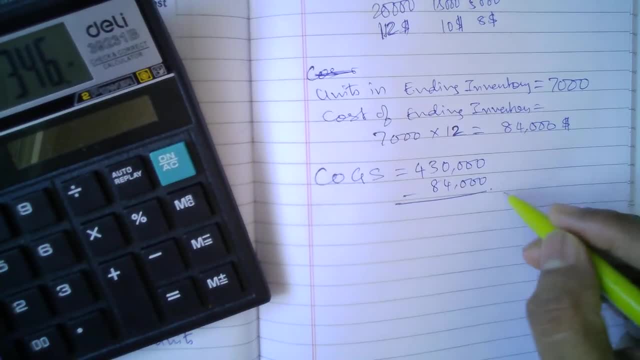 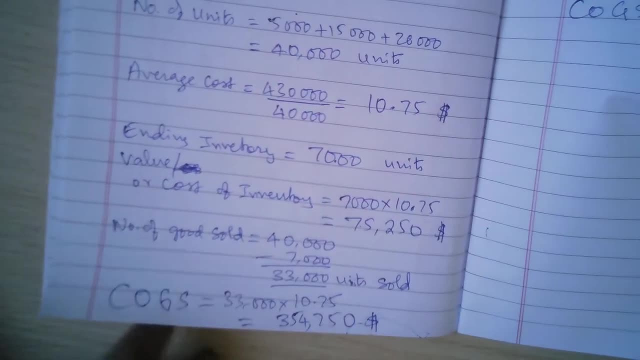 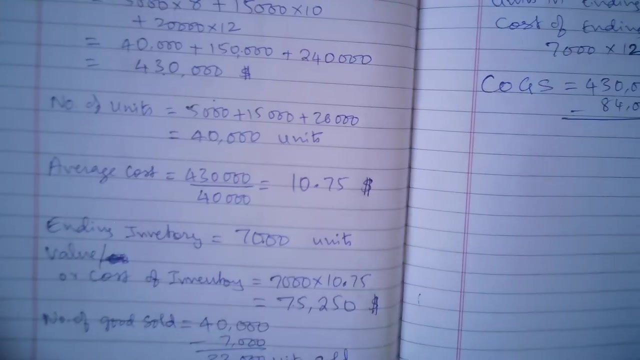 So 430000.. thirty minus eighty four, so three forty six. three forty six thousand dollars is the cost of goods, whereas here, if you see, the cost of goods sold is less. so here cost of goods sold is more okay. so like that it will be the difference. okay, now let us do last in. 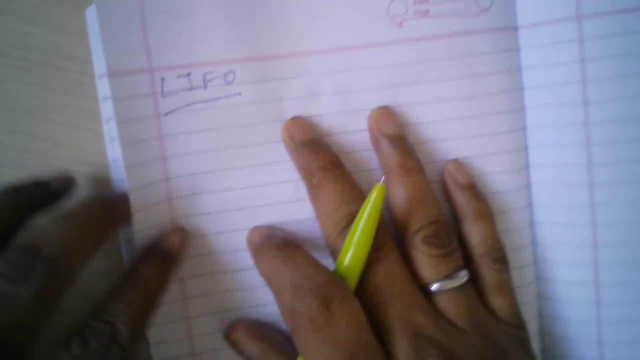 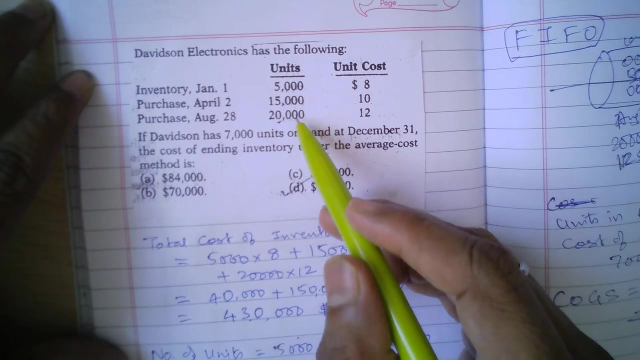 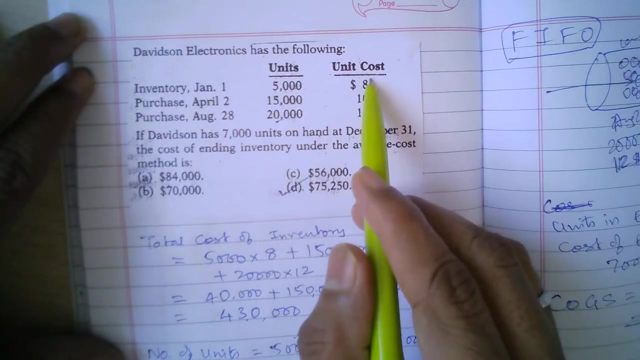 first out. okay, so if you go for LIFO, last in, first out. so which was the lead recent one? this twenty thousand, this is the lasting, so this is already sold. this is sold like that. so what is left in the inventory? seven thousand units, but here five thousand units. 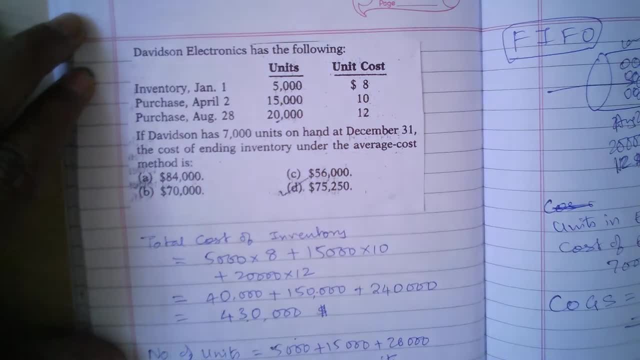 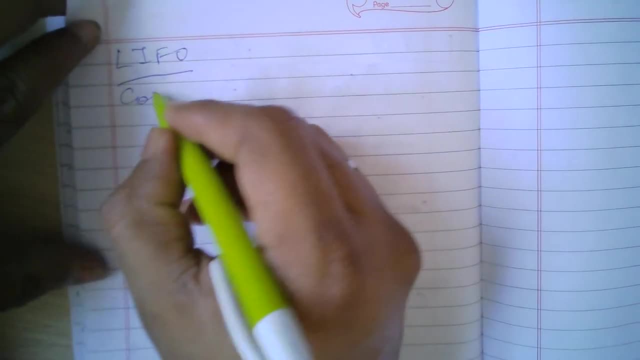 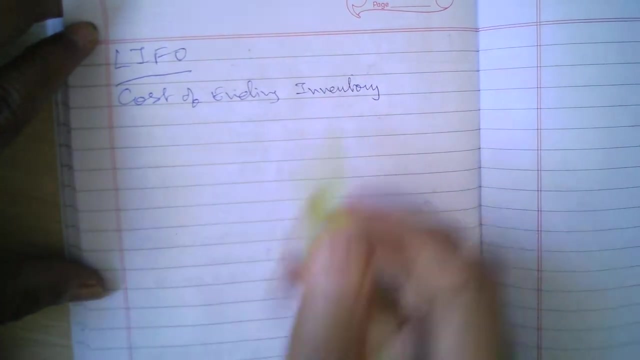 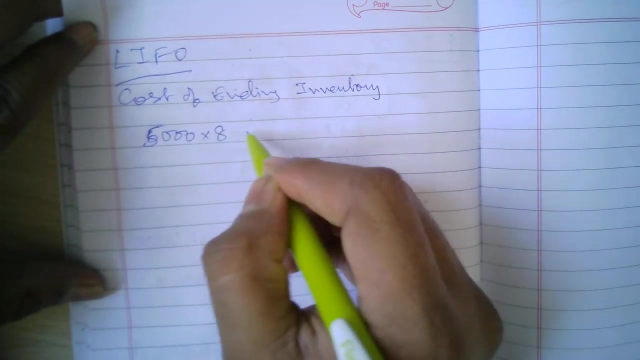 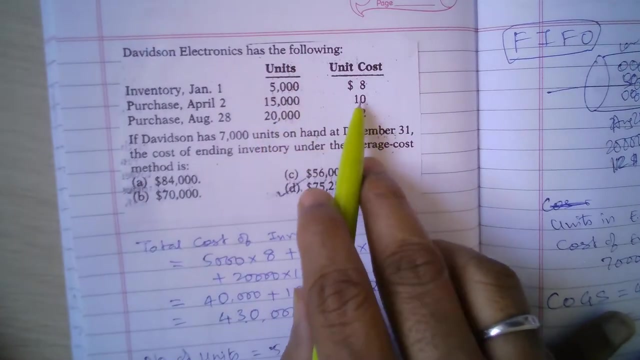 are costing eight dollars. seven thousand is more, so out of the seven thousand, the first five thousand will be at eight dollars. okay, so so here, cost of ending inventory. so cost of ending inventory: what I will get will be 5,000 at 8 dollars plus 2,000 at what was the next group, 15,000 in that. out of this, 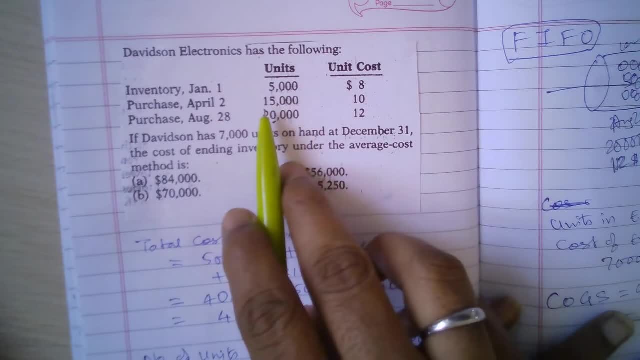 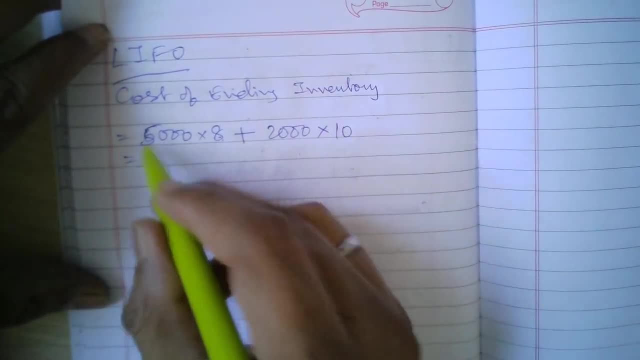 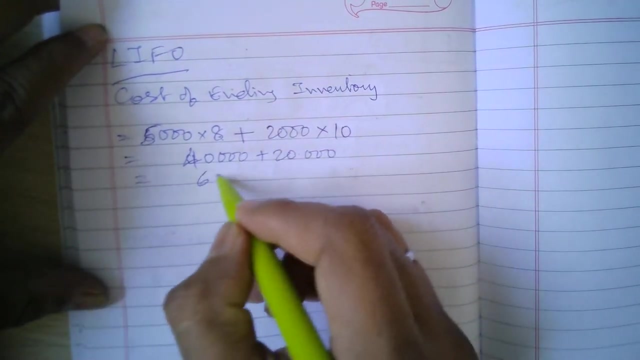 15,000, 2,000 will be retained and remaining 13,000 are sold and remaining 20,000 are sold. So only 10, 10 dollars here into 10.. So here 8 into 5 is 40,000 plus 20,000, so that is 60,000 is the cost of the ending inventory. 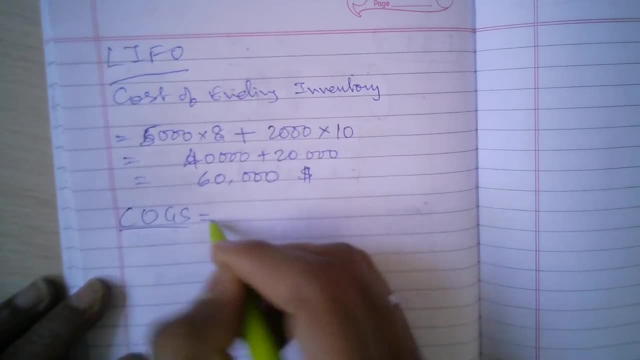 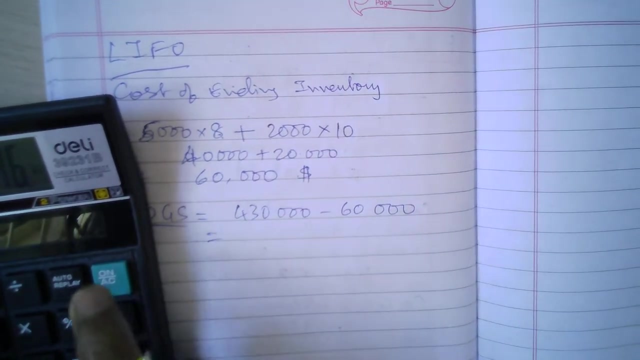 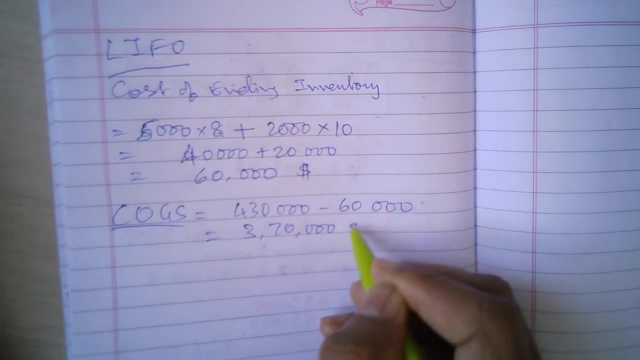 So therefore, what is the cost of goods sold? COGS, So cost of goods sold will be 43,000 minus 60,000.. So we will get 430 minus 60. So 370 dollars. Okay, So let us compare okay. 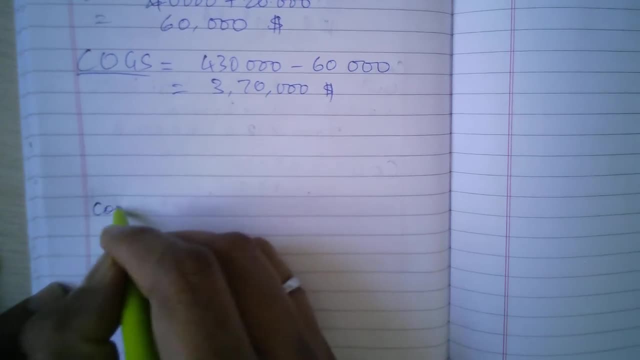 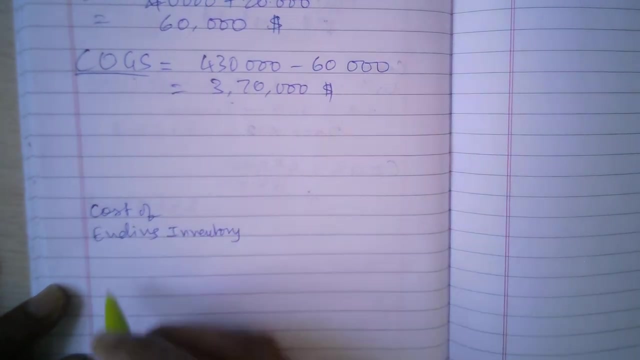 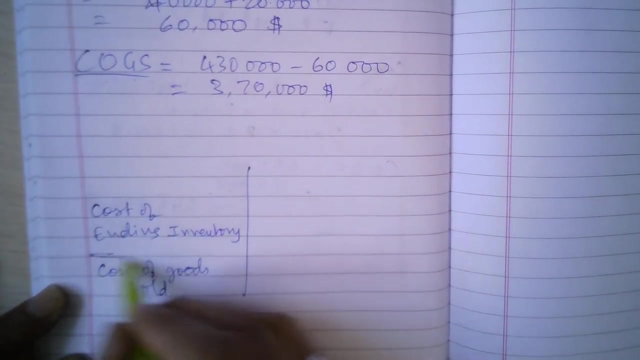 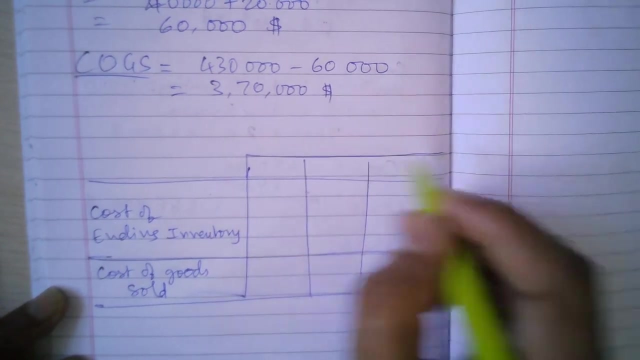 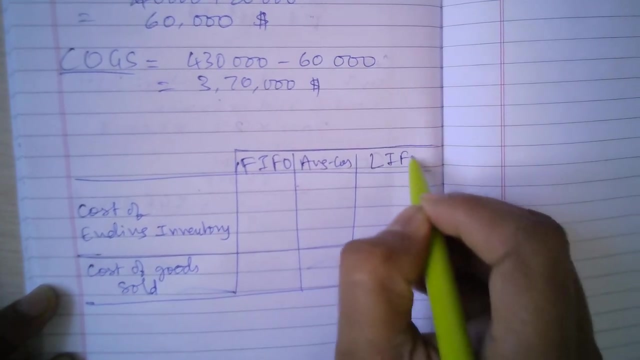 So what we are comparing is cost of ending inventory, cost of goods sold. So what are the three methods? So first method is FIFO method, first in first out. Next method is average cost method and LIFO method. Okay, So why I kept average in middle is that the answer will be in the middle of these two. 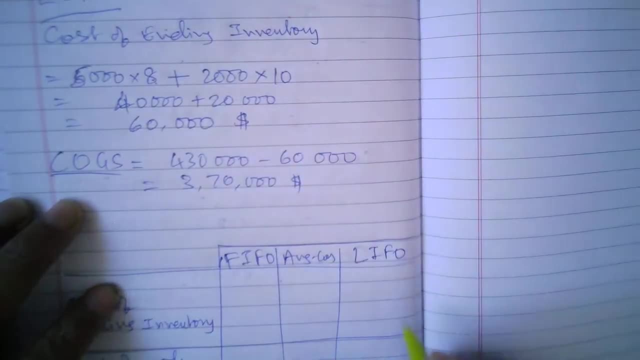 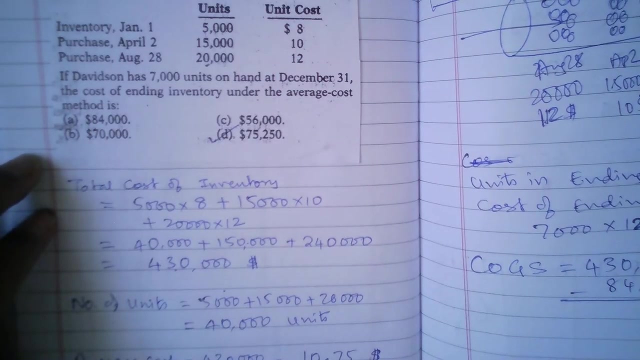 Okay, So you see the. for the LIFO method, 60,000 is the cost of ending inventory, Whereas in the FIFO method the cost of ending inventory is 84,000.. And whereas the average cost method the cost of ending inventory is 84,000. 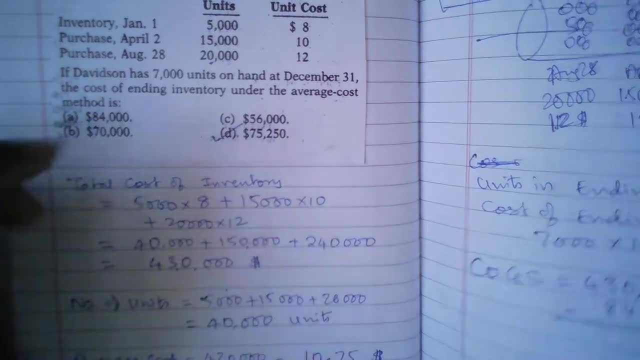 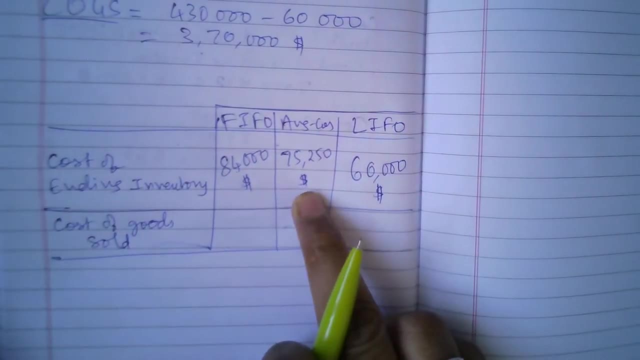 So the cost of ending inventory is 84,000.. Okay, So the cost of ending inventory is 75,250.. So now you can see this is high, this is next higher and this is lower. So for the same amount of inventory you are getting different results. 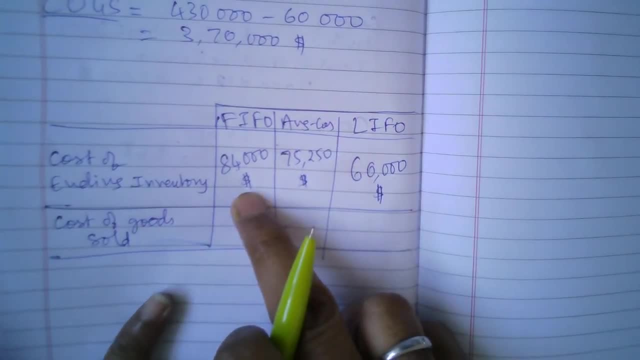 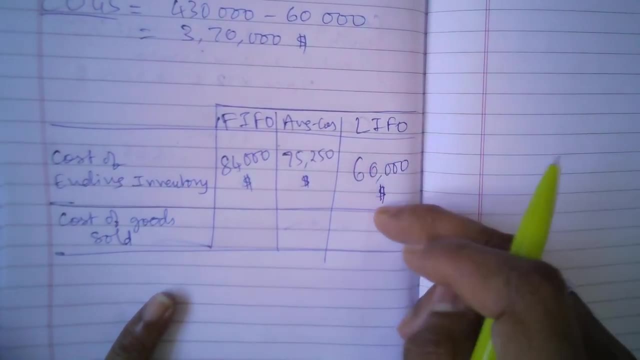 So obviously the cost is changing. So if the cost is more, profit will be less, And if the profit whereas if the cost is less, the profit will be more. So you may think that, okay, profit is more, So let us go with LIFO principle. 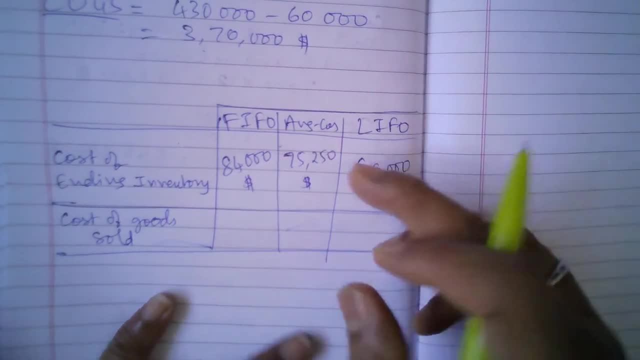 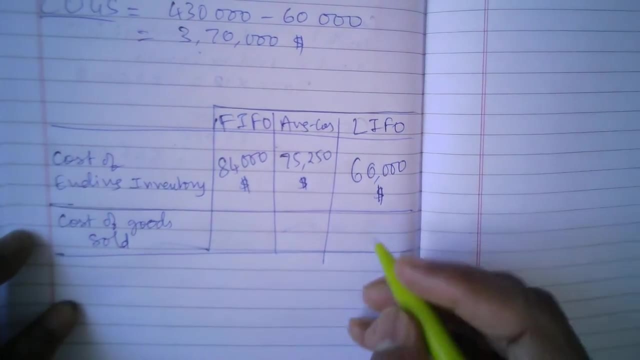 But then we have to understand that the profit value will be less. So if your profit is more, income tax will be more. So it is not always that you have to go for one method or the other. it is the company decision. Similarly, cost of goods sold. here it is 370, whereas in the average cost method it.